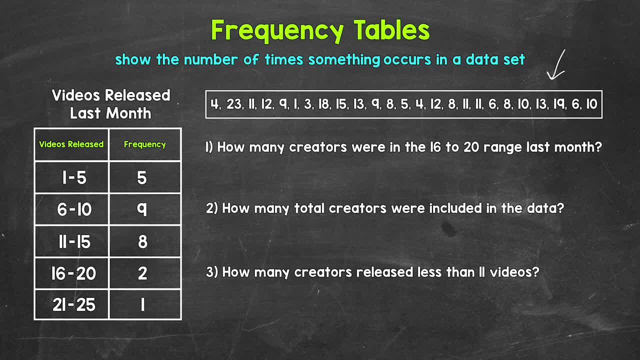 month by a group of content creators, so a certain number of creators were asked about the number of videos they released last month. These are the results. Now, this is raw data. That just means that this is the data as it was collected. It's not organized at all, so you can. 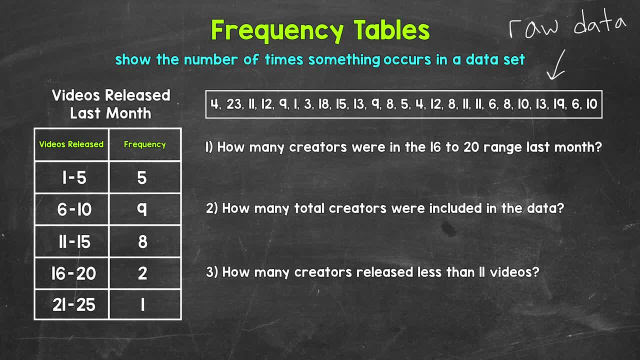 see it's difficult to interpret, as is A frequency table will help us organize everything and our table is right here to the left. Now the left column of the table. so this column going down right here, that's the number of videos that were collected last month. So this is the number of 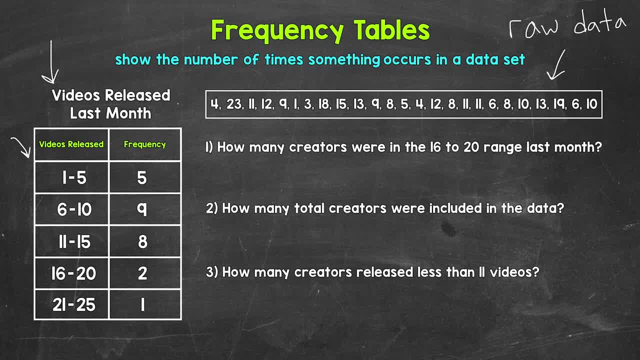 videos released. So we have 1 to 5 videos, 6 to 10 videos, 11 to 15 videos, 16 to 20 videos and then 21 to 25 videos. Now these groups are called classes or class intervals. Since we have these, 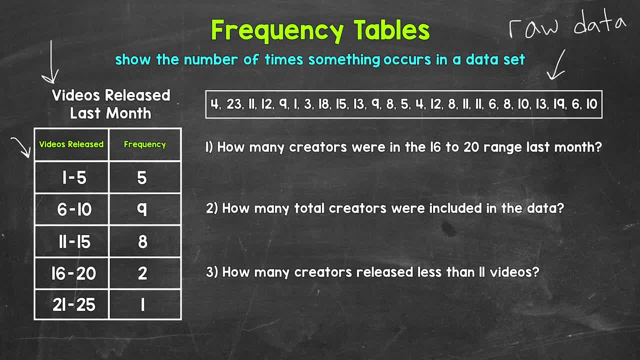 classes, these groups. this is called grouped data, So these are the groups right here in the videos released Column. If we have a wide range of data and a lot of individual values, using groups helps us create a more condensed and manageable table, Depending on the situation and the data writing each. 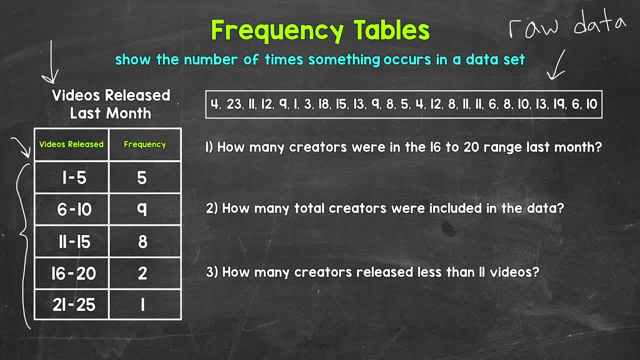 individual value could create a very long table. For example, for this data we would have to go from 1 to 23.. That table would be pretty long. So think about if we had an individual table and if we had an even wider range and more individual values, maybe hundreds or even thousands of. 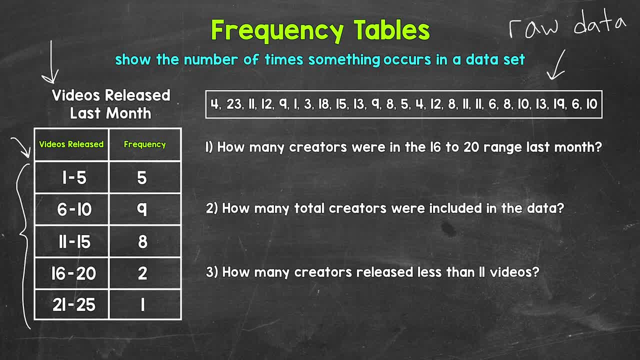 values. So these groups allow us to create a simpler and easier to work with table. Now, as far as the right column, so this column right here. this is the frequency, the number of times the values in our data show up within these groups. So, for example, taking a look at the table, we have a 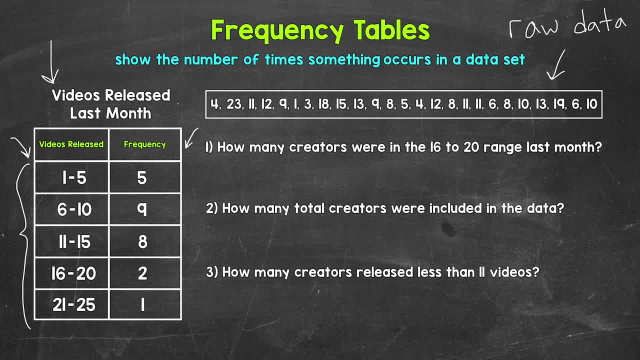 frequency table And reading this table, how many creators released 1 to 5 videos last month? Well, 5 creators. How about 6 to 10 videos? Well, 9 creators. 11 to 15 videos. 8 creators 16 to 20. 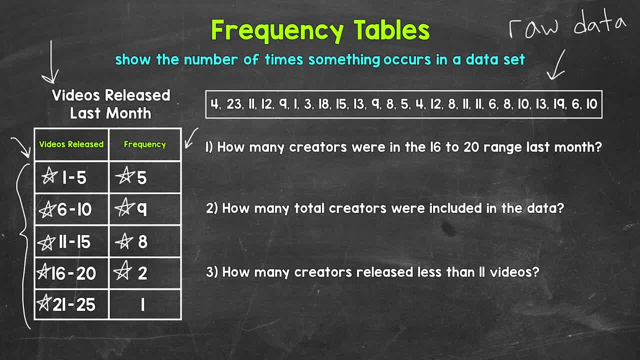 videos 2 creators And then 21 to 25 videos- 1 creator. So you can see that this frequency table really helps us create a more consistent table. So if we have a wide range of data, we would have to. 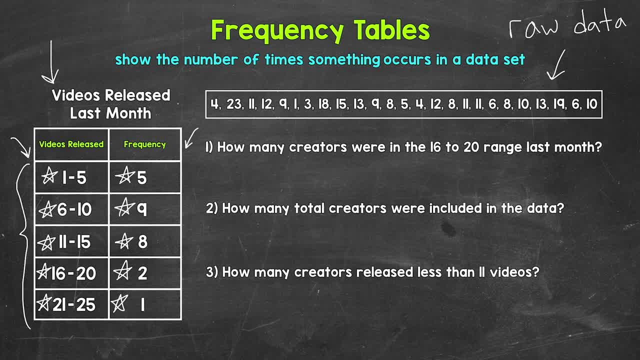 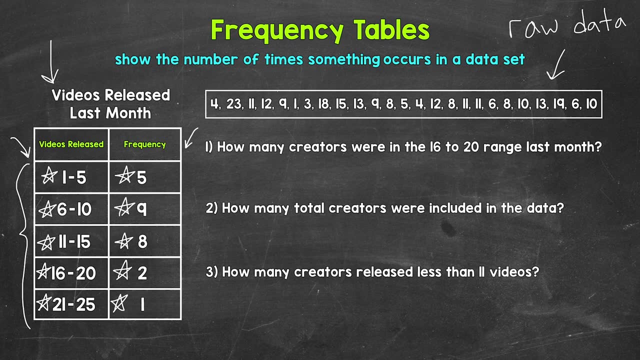 really help organize and present the data in a more meaningful and easier way to look at than just looking at the raw data. Now let's answer some questions regarding the data, Starting with number 1, where we have how many creators were in the 16 to 20 range as far as videos released. 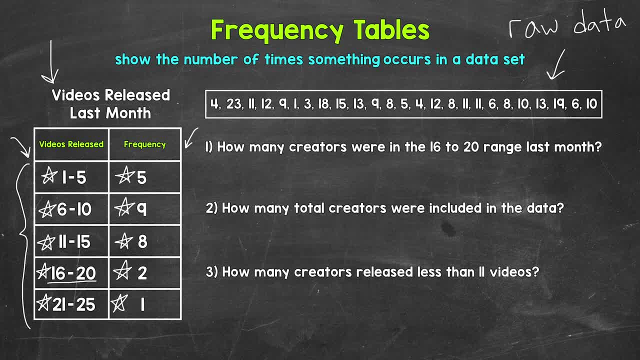 last month. Here is 16 to 20 right here, So we have 2 creators. 2 creators released 16 to 20 videos last month, So they were in that range. Let's move on to number 2,. 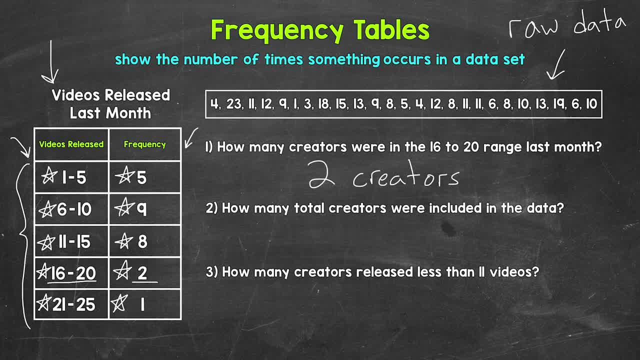 where we have how many total creators were included in the data. Well, for this we need to take a look at the frequency column and add all of those numbers up. So we have 5 creators, 9 creators, 8 creators, 2 creators and 1 creator. 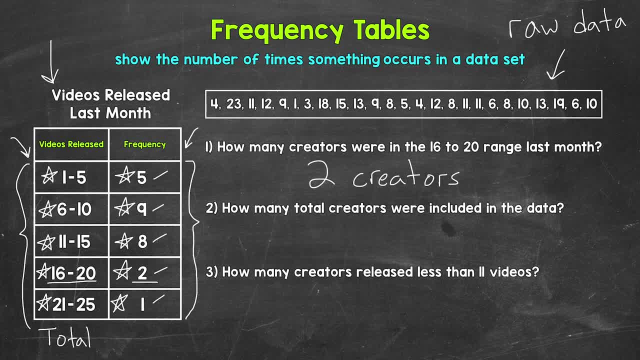 So if we add those up, that's going to give us the total amount of creators. Well, 5 plus 9 is 14, plus 8 is 22,. plus 2 is 24, plus 1 gives us 25.. So 25 total creators. 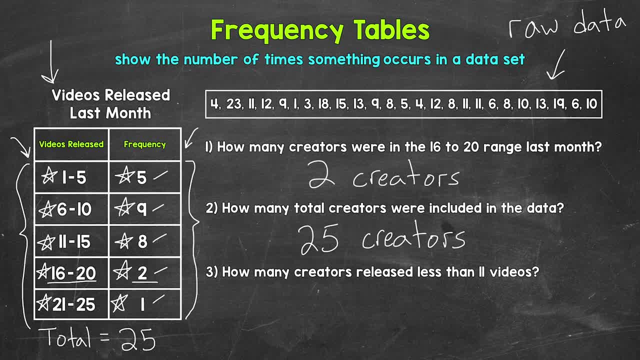 And then, lastly, let's move on to number 3, where we have how many creators released less than 11 videos. So less than 11, 11 is not included, So we are going to look right here. So the 6 to 10. 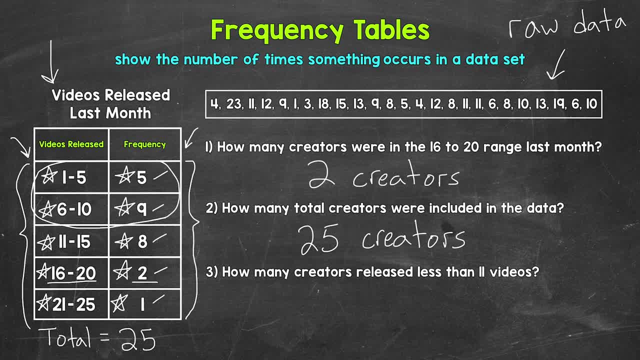 and the 1 to 5 videos released. So we have 5 creators and 9 creators. So 5 plus 9 gives us 14 creators released less than 11 videos last month. So there you have it. There are the basics of how to read and understand frequency tables. 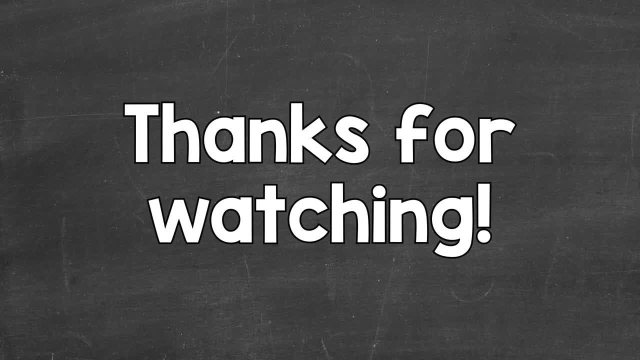 I hope that helped. Thanks so much for watching. Until next time, peace.